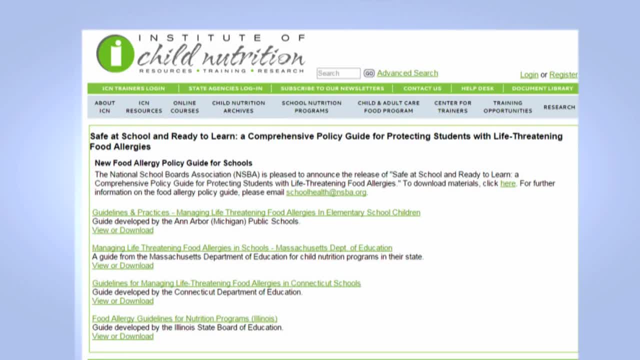 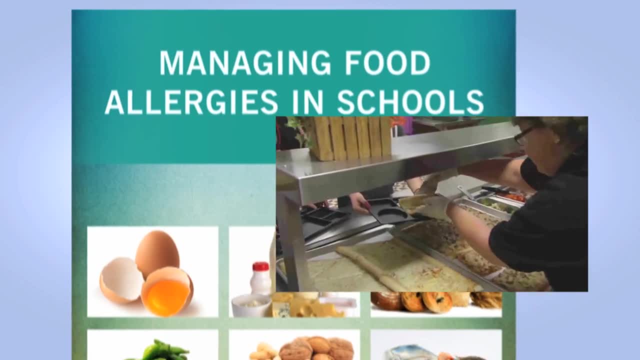 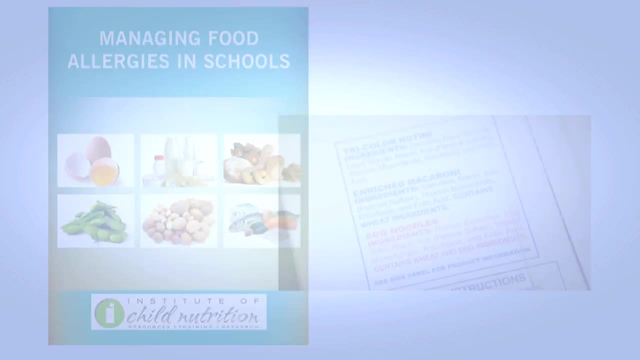 The Institute provides a variety of resources related to managing food allergies in schools and child care, such as videos and fact sheets, including information about specific allergens, standard operating procedures and links to other useful resources. Additionally, the Institute has face-to-face training and an online course on how to manage food allergies in schools. 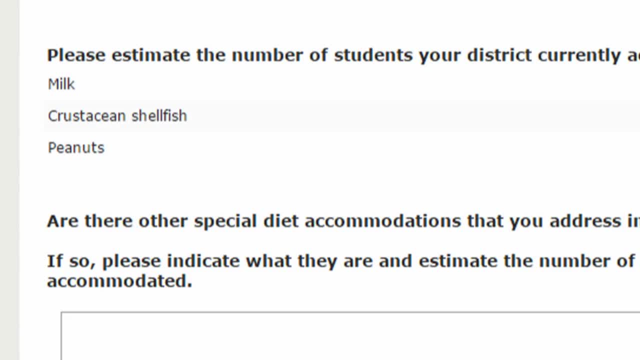 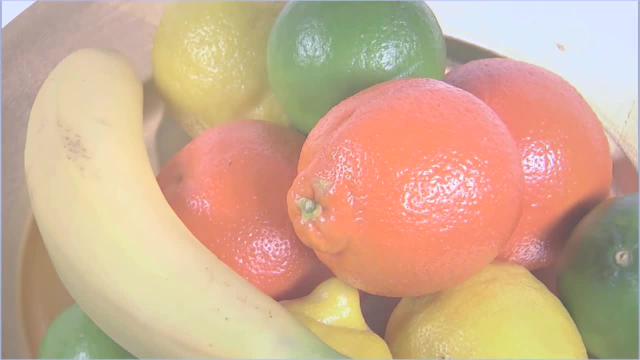 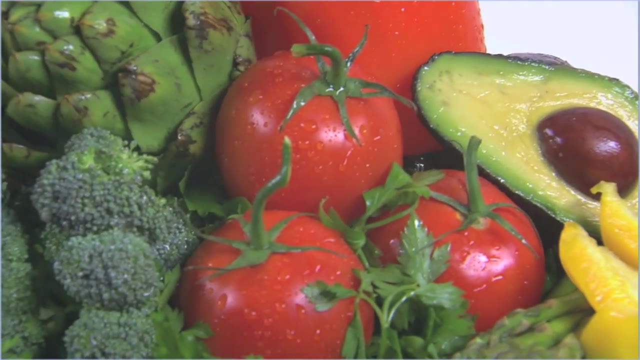 The Center of Excellence completed a national survey on food allergies. A second example is produce safety. Many fruits and vegetables are eaten fresh or raw and don't include a cooking step that will kill pathogens and prevent illness. The USDA deems it such an important topic that they have partnered with USDA's Agricultural Marketing Service. 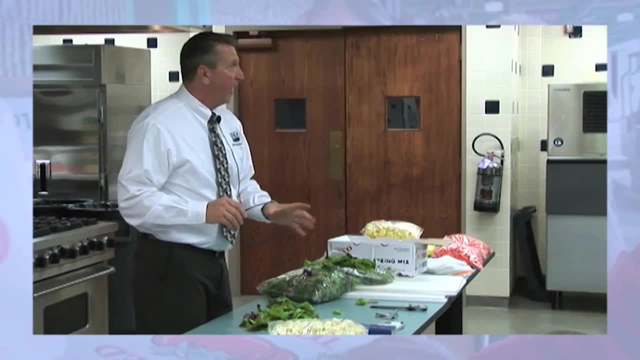 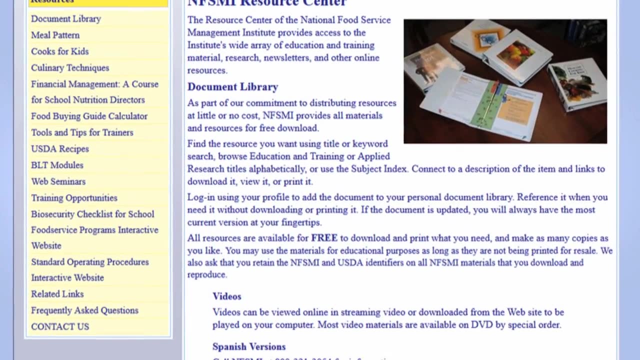 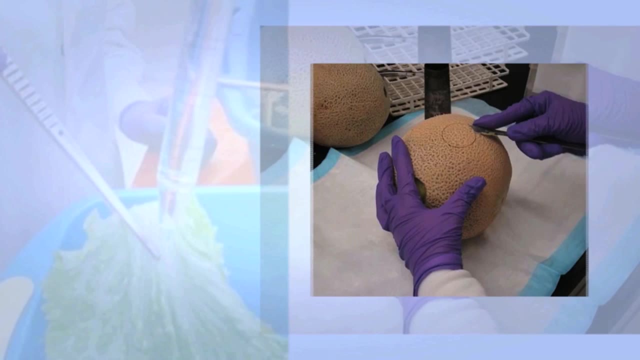 to offer Produce Safety University, an educational program that has reached over hundreds of participants. The Institute offers best practice resources, fact sheets, PowerPoint presentations and videos that address produce safety, And the Center of Excellence has conducted preliminary research on the effects of different produce wash methods. 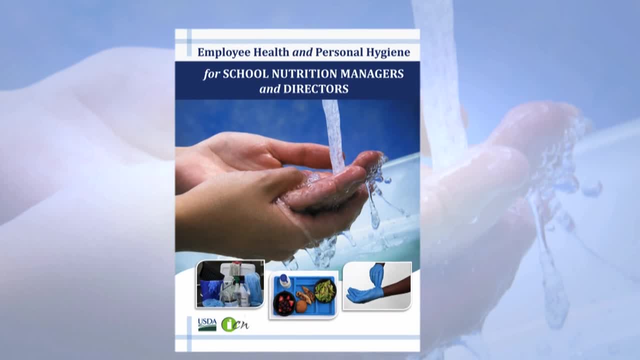 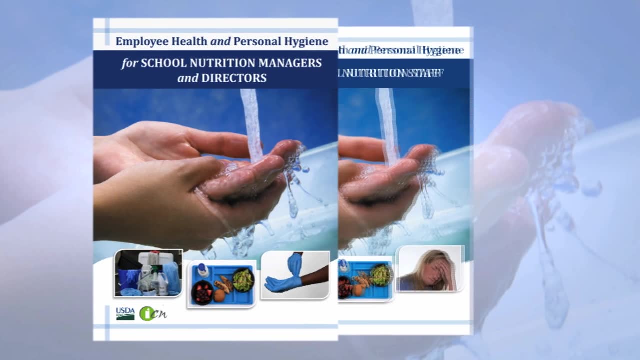 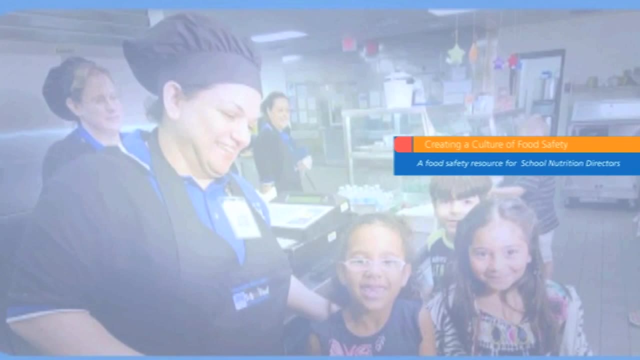 The Institute addresses the topic of employee health with the release of the Employee Health and Personal Hygiene Guide for school nutrition managers and directors, as well as guides for employees in school nutrition and child care. Creating a culture of food safety is being addressed in a variety of ways. 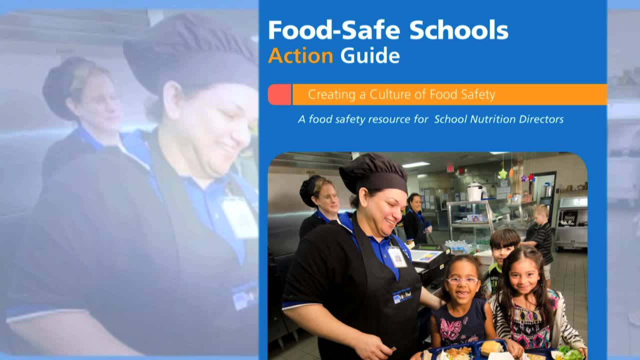 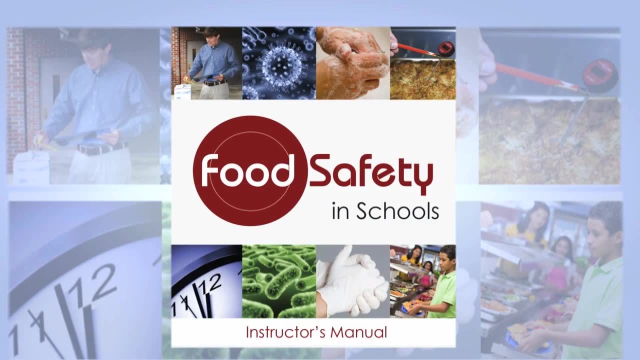 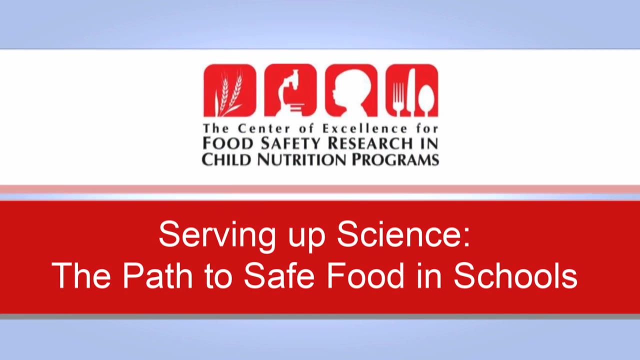 The USDA published the Food Safe Schools Action Guide and the Institute has updated Serving It Safe, which is now called Food Safety in Schools and is available in Spanish. The Center of Excellence offers Serving Up Science: the path to safe food in schools. This week-long program focuses on the scientific principles behind food safety. 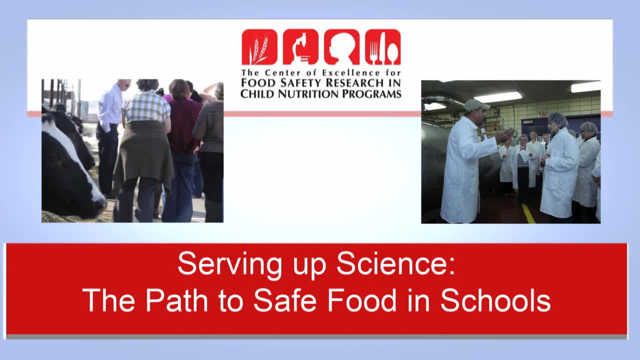 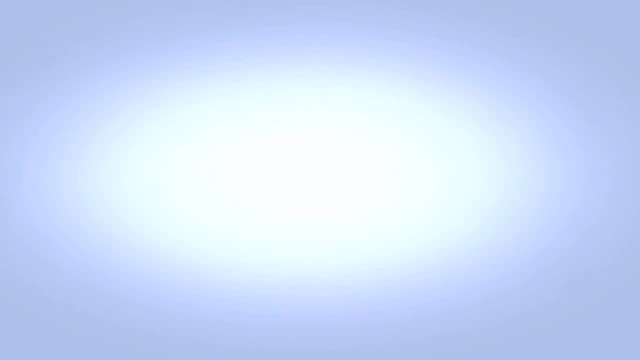 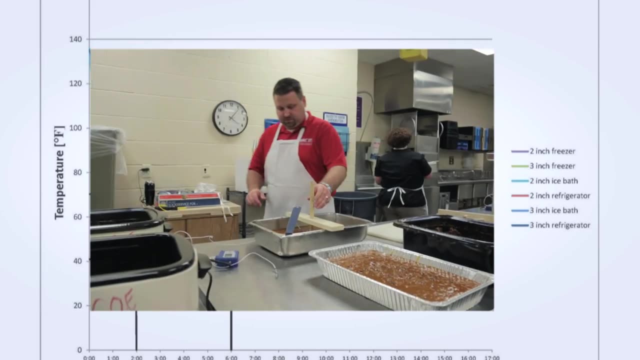 and provides school nutrition leaders with tools to help improve food handling practices and methods to foster a culture of food safety in schools. The Center has research initiatives focused on impacting behavior, reducing wasted food and simulating temperature and microbial growth for meals served outside the school cafeteria.